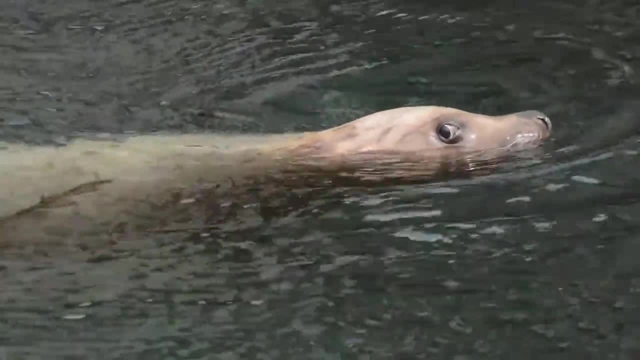 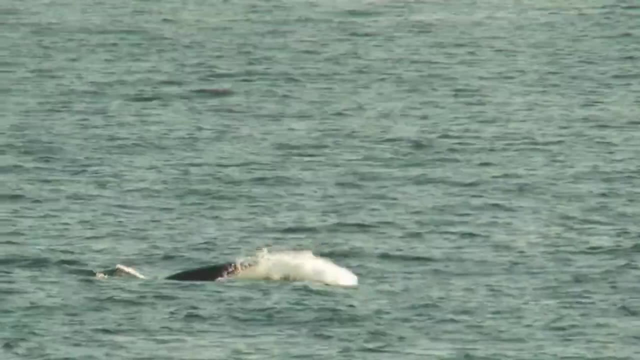 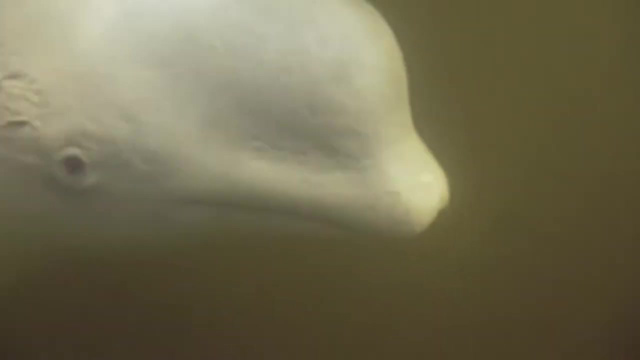 healthy again. There have been some success stories. For example, the eastern population of stellar sea lions and the eastern North Pacific gray whale have recovered and were removed from the list. But there are other species that are struggling. Of all the species we protect, we consider some to be among the most at risk of extinction in the near future. 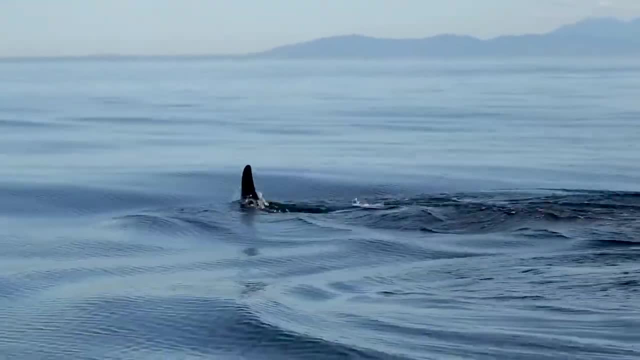 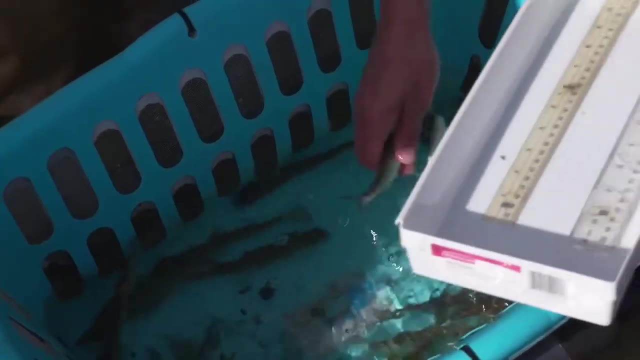 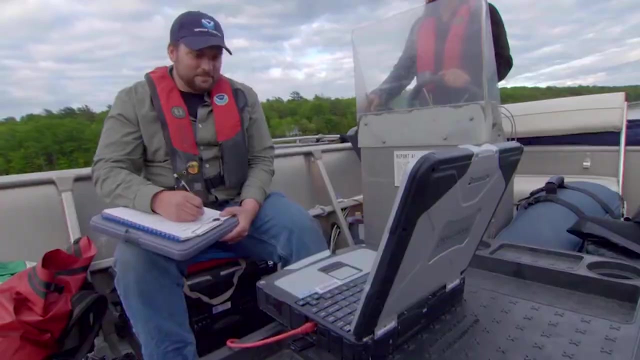 That's why, in 2015,, we created the Species in the Spotlight initiative. It's a way for us to focus our time, energy and resources on these at-risk species and bring greater attention to their plight. Our goal is to focus our recovery actions and motivate partners. 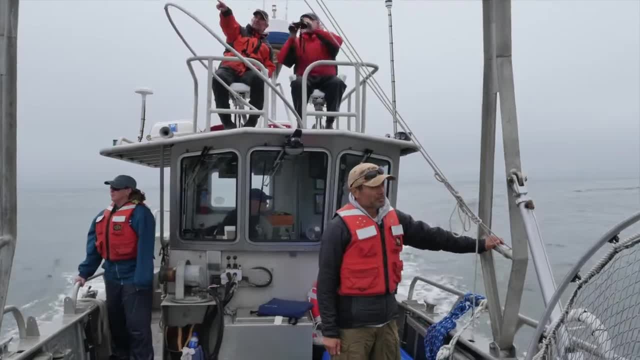 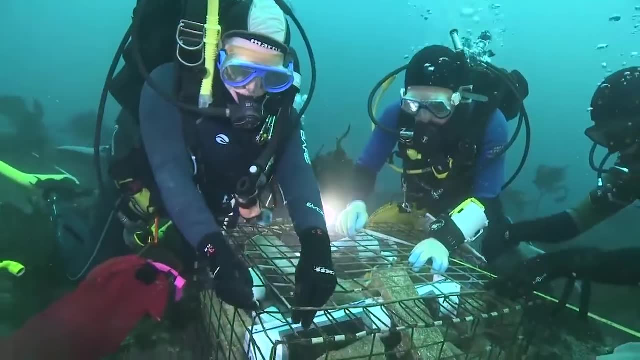 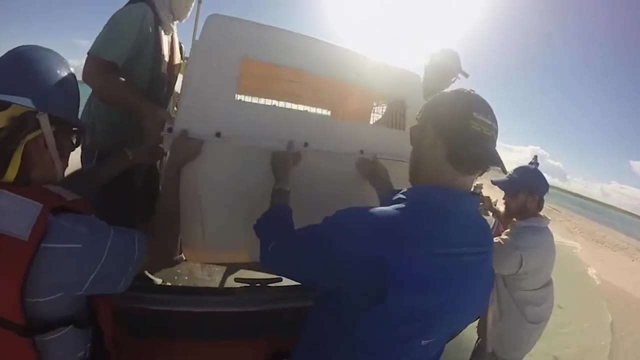 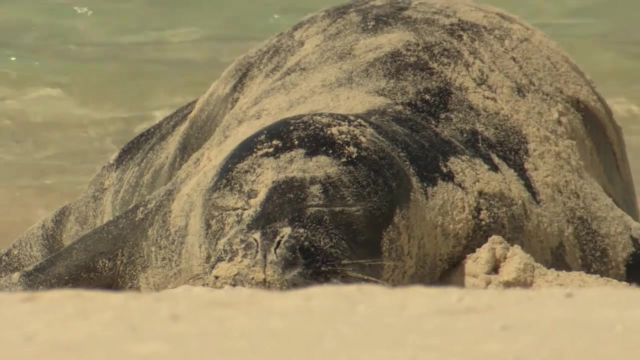 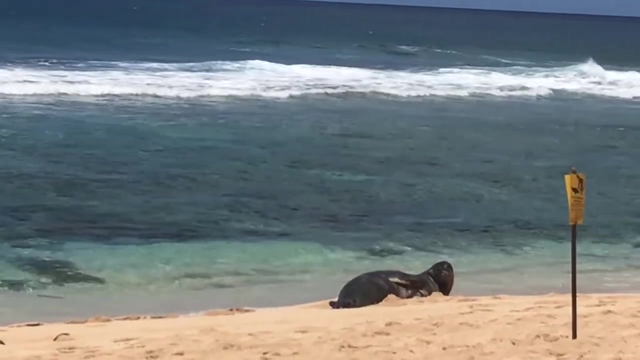 and community members to work with us on these actions. In the first five years of the Species in the Spotlight Initiative, we have made real progress toward stabilizing some populations, such as Hawaiian monk seals. We launched the first-ever effort to vaccinate a wild population and have vaccinated more than 700 monk seals. 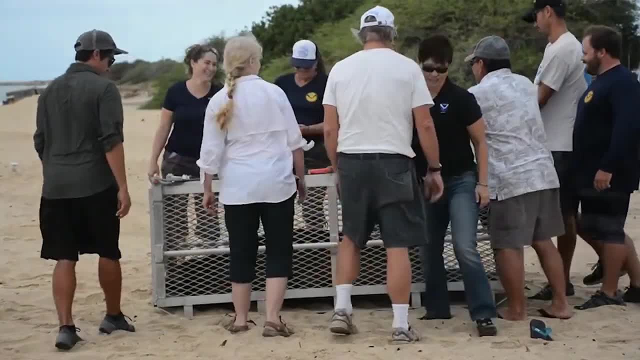 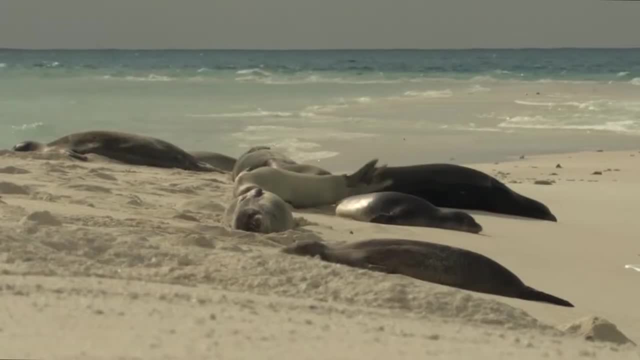 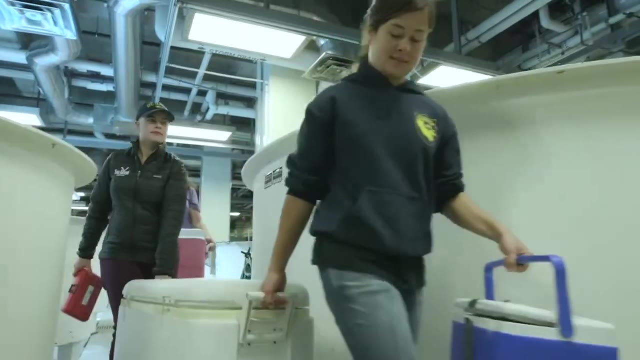 We also partnered with local organizations to rescue and rehabilitate more than 150 animals. Our recent data shows that their population appears to be slowly increasing. Sometimes, the only way to bring back a species is through captive breeding. We are doing this successfully with white abalone. 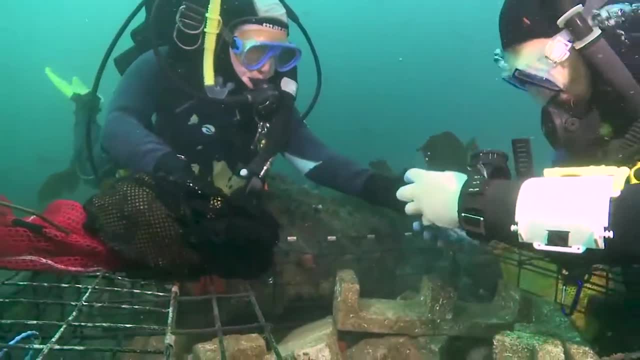 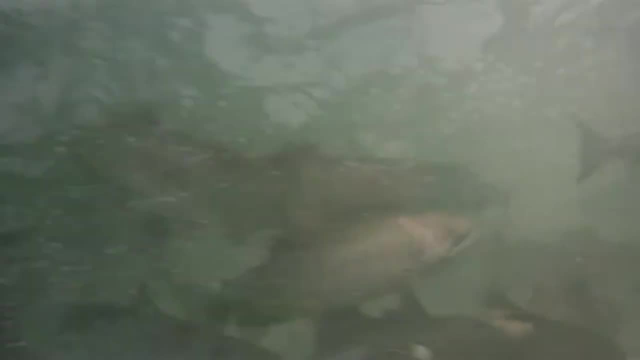 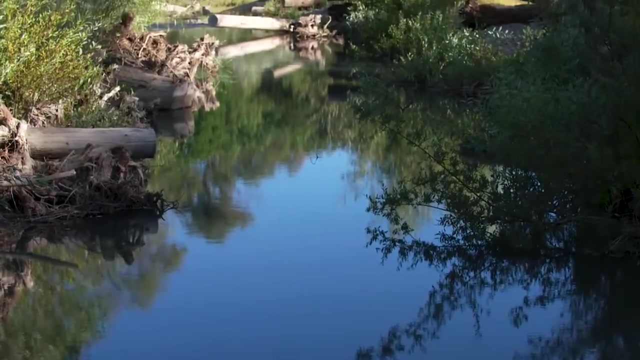 and just started planting thousands of young abalone into their native habitat. We also reintroduced approximately 560,000 winter-run Chinook salmon to establish a new population in Battle Creek in California. We also focus on protecting the habitat and prey that these species need to recover. 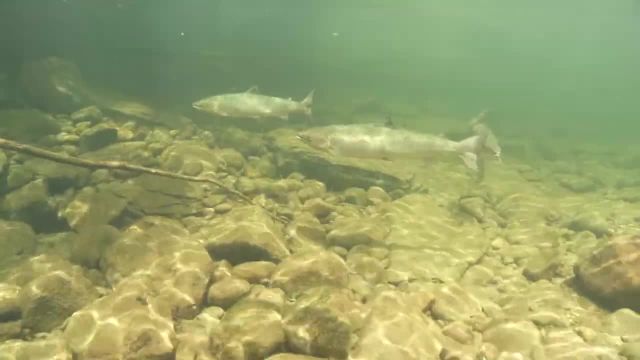 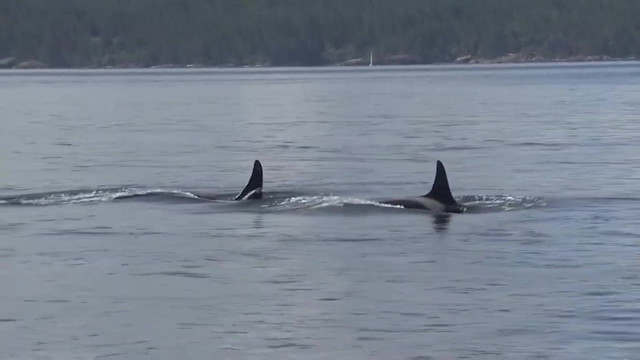 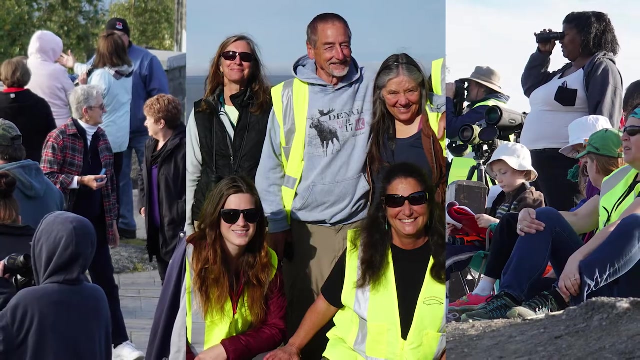 such as removing dams from rivers that block Atlantic salmon from reaching spawning grounds in Maine, protecting Chinook salmon stocks that southern resident killer whales need for food and restoring more than 200 miles of streets for coho salmon. An important part of our work is to educate and engage people. 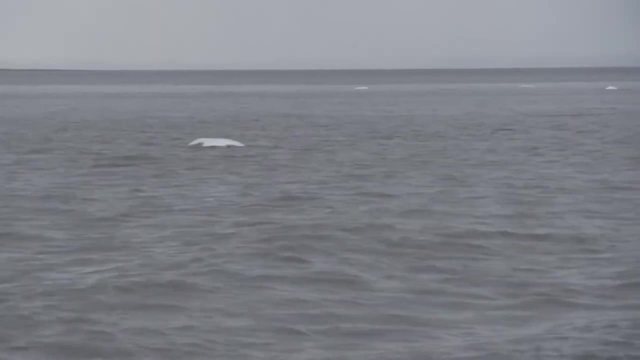 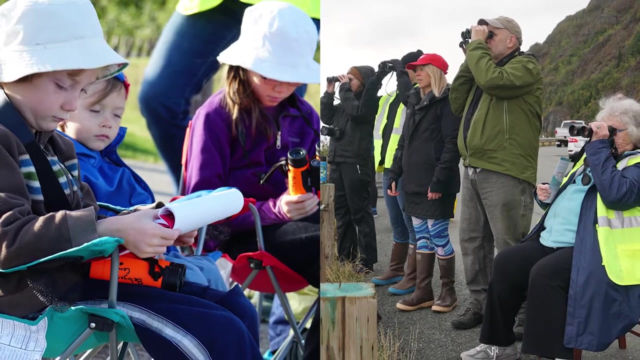 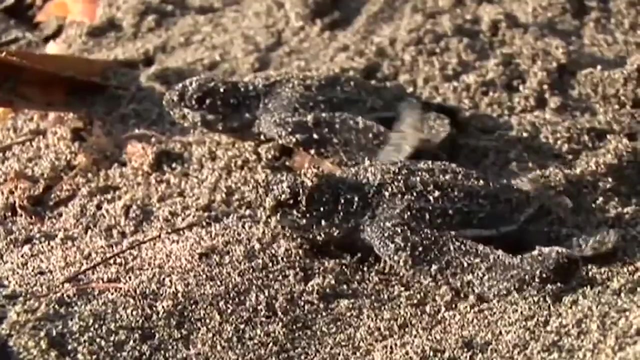 who live, work and play near these endangered animals. Hundreds of people participate in our annual Belugas Count Day and our Alaska Beluga Monitoring Partnership, helping scientists get more information on Cook Inlet beluga whales, And we have worked with community groups to protect key leatherback sea turtle nesting beaches.